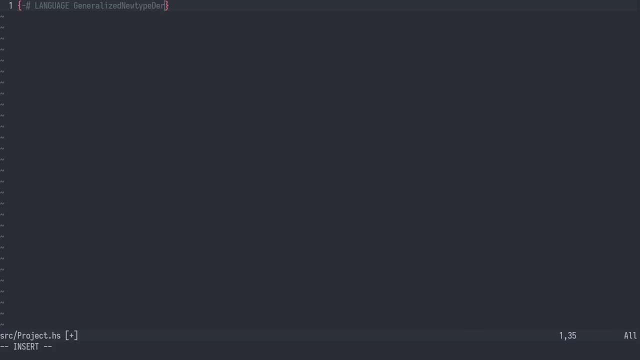 hold our core data structures. We need to enable the generalized new type deriving for new types. We say that this is the project module and we import the text type. We'll be working with money, so we create a new type around a double We. 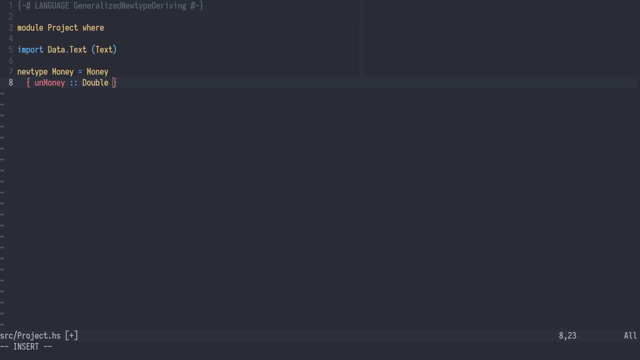 call the field unMoney to be able to unwrap it. We derive instances for show, eek and num. The same goes for our project ID type. It's a new type wrapper around an int and it also derives show, eek and num. The central data type in the system is the project. 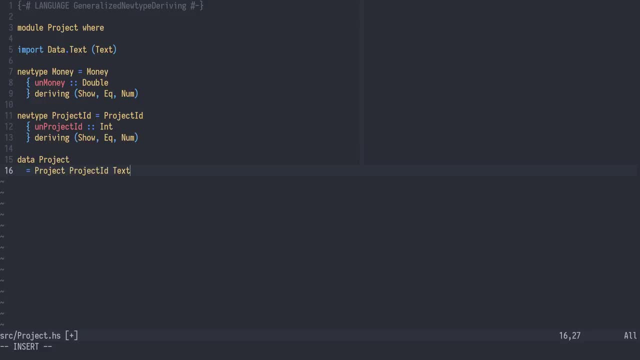 which is either a single project with an ID and name, or a project group which has a name and a list of sub-projects. This type also derives show and eek. The budget data type holds two fields: the income and the expenditure of the budget. 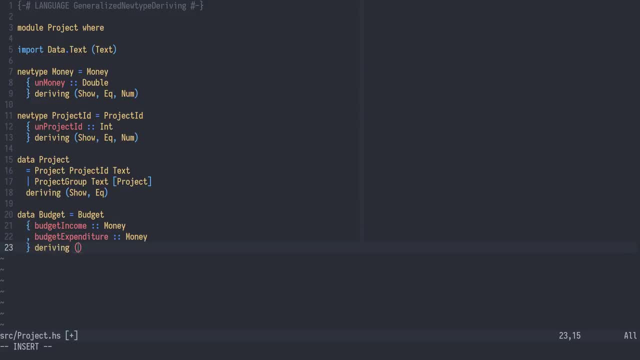 A transaction is a very simplified model which is either a sale of some money or a purchase of some money. Let's format and save this file. Let's open up the demo module. I'm using this for imports in the REPL, so I'll turn off the warning about unused imports. Also, we 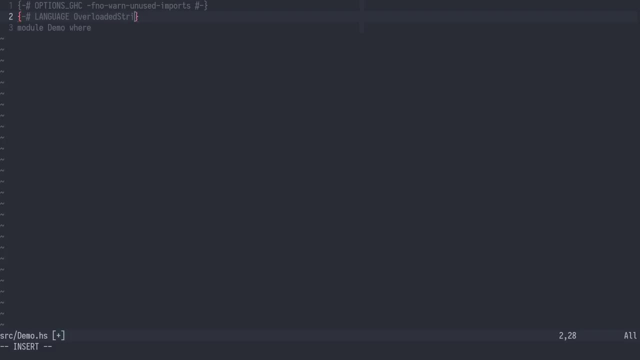 need to overload the strings language extension. Now we'll import our project module and start writing some data based on our project. Now we'll import our project module and start writing some data based on our project. Now we'll import our project module and start writing some data based on our project. 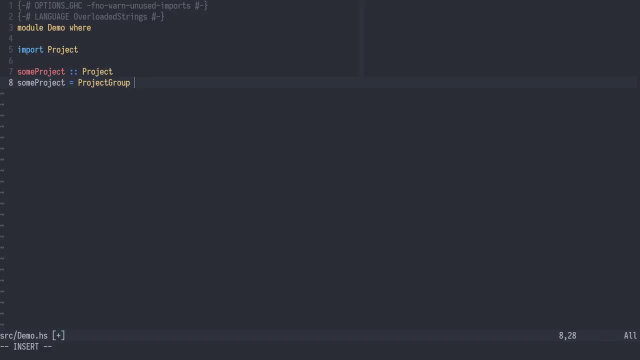 This is a project defined as a group called Sweden, which has three sub-projects: Stockholm, Gothenburg and Malmo. The domain model is very generic so far, and here I'm using it to model something location based in Sweden, like construction sites or something. 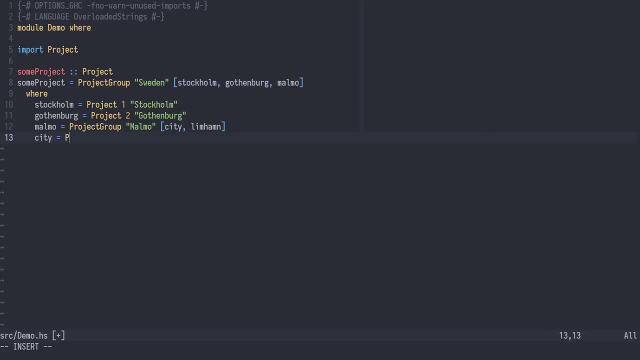 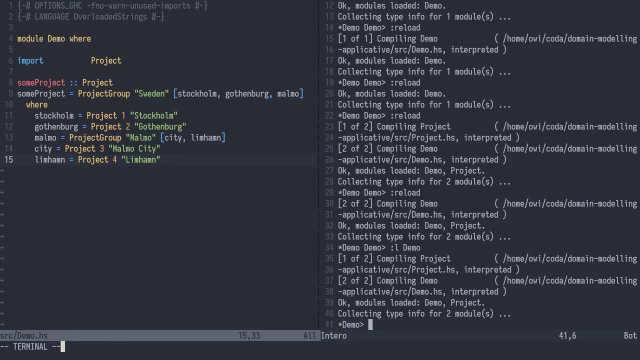 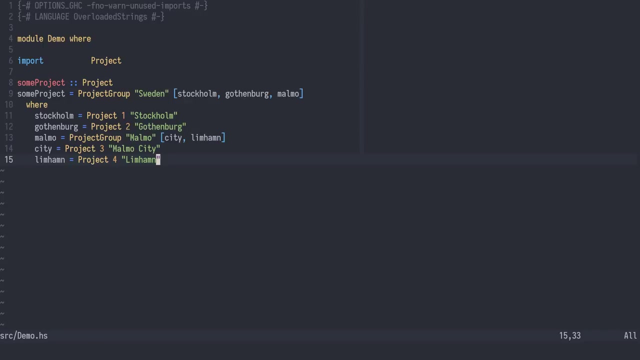 Okay, we now have some data. we can try it out in the REPL. We'll simply evaluate the SUMPROJECT and see what it is. Yeah, it works, But now the customer wants some reporting. based on this, We'll create a new module called database, where we will implement some fake queries. 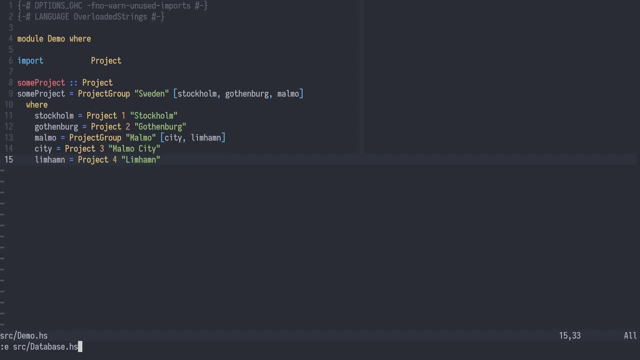 to work with. In a real system. these would likely be database queries To generate some fake data. we'll use the SYSTEM RANDOM module. We'll also need our PROJECT module and then we can start writing a query for budgets. It'll be a function from PROJECT ID to an IO action of budget. 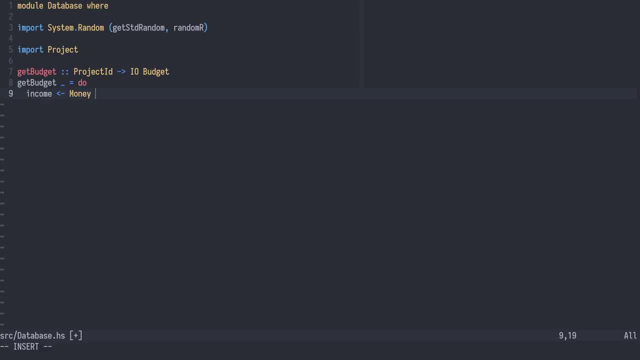 Ignoring that PROJECT ID And simply generating some money within the range of zero and ten thousand. The same goes for expenditure, And then we will construct a budget value. The next query is: GET TRANSACTIONS From PROJECT ID to an IO action. 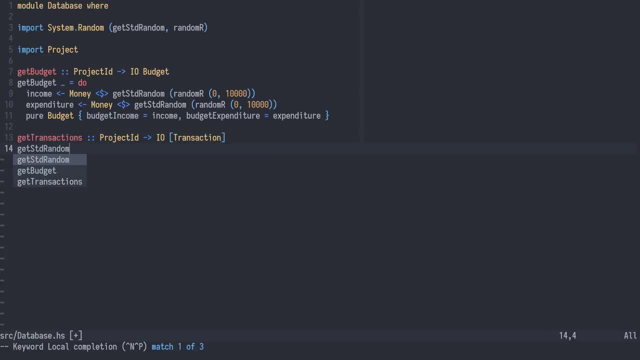 Of a list of transactions. It also ignores its argument and constructs random data. A sale of some money within the range of zero and four thousand. The same goes for a purchase. Then we return the sale and the purchase in a list. We can now go ahead and implement our reporting module. 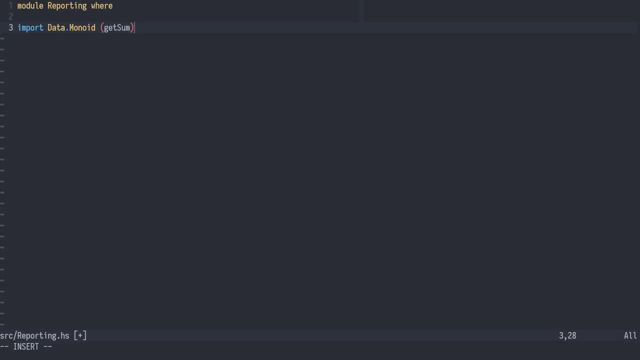 We'll import the GETSUM function from DATA MONOID And we'll import our own modules, database, qualified as DB and project. A report is a data structure of three fields: The budgeted profit, The actual net profit And the difference between the two. 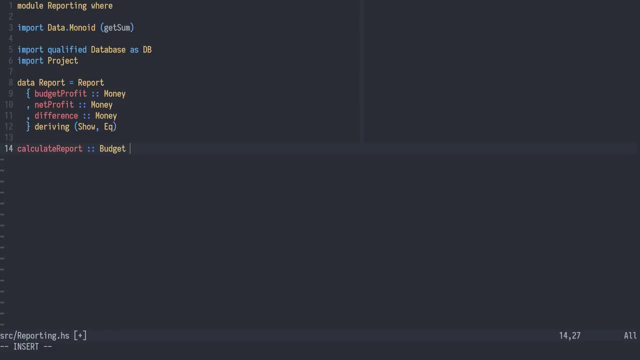 We create a pure function called CALCULATE REPORT From BUDGET to LIST OF TRANSACTIONS. to REPORT, It takes a budget in the transactions And creates a report value. We will reuse some of these values, So I'll create prime named versions of them in a WHERE block below. 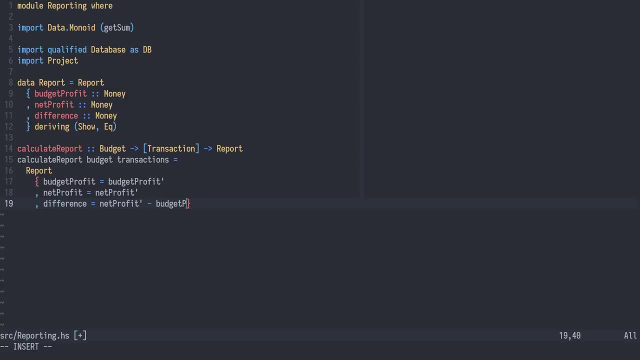 But the difference is calculated from the net profit prime And the budget profit prime. The budget profit is defined as the difference between the budgeted income and the budgeted expenditure. The net profit is defined as the sum of the profit of all transactions. 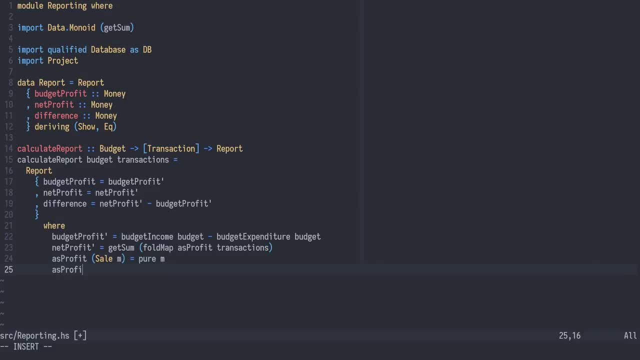 A sales transaction is considered a profit And a purchase is negated. We'll now use our fake DB queries to calculate a report for a project, The function from project to an IO action of a report. It's defined with the CALC function. 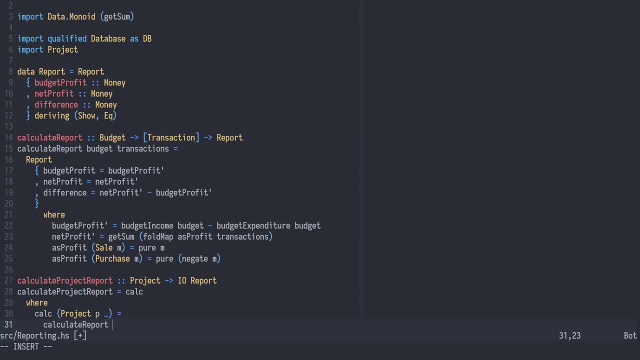 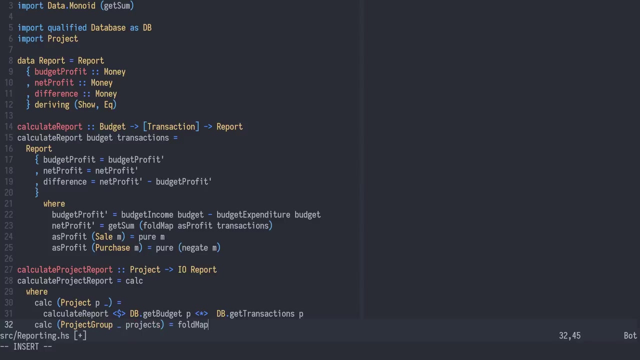 Which, given a single project, will use our pure CALCULATE REPORT function over the results of the GET BUDGET Get transaction queries. Given a project group, it will fold over the projects using the CALC function. For this to work, we need a monoid instance for REPORT to be able to concatenate them. 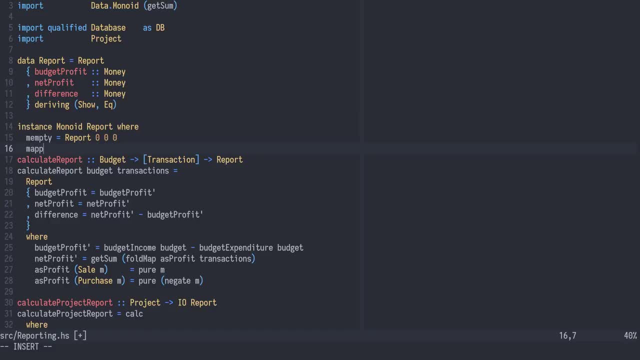 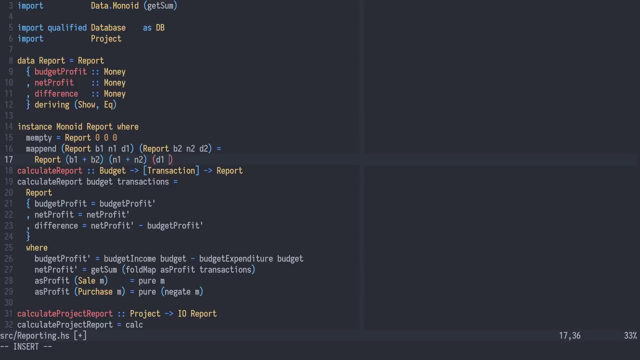 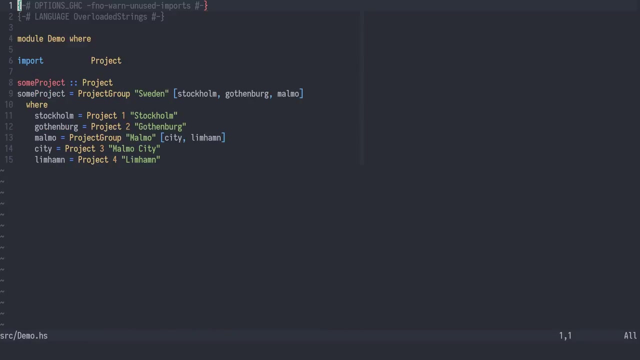 The empty element is a report with zero for all the field, The MAPPEND implementation. We'll take the budgeted profit, the net profit and the difference And sum them up. Let's go back to the 데모 module and try that out in the REPL. 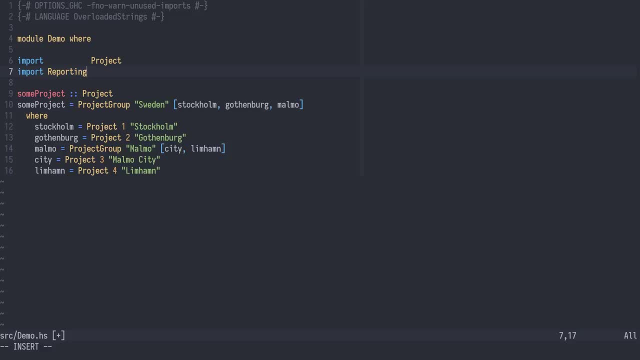 We import the reporting module And open the REPL. Given that we have a project, We can use this reporting module and REALLY late andonsックudrycom to do also true reporting. A supplier is holding costs directly to your machine. We can calculate a project report. 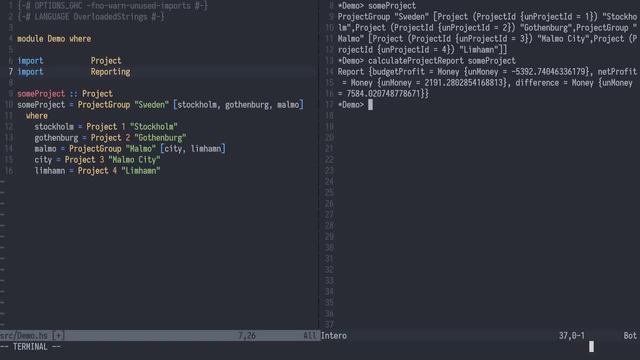 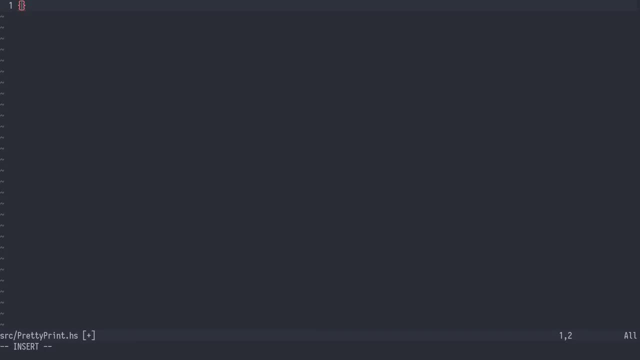 There we go nice, But we would like to format this a bit nicer. We create a new module called PrettyPrint. Inside a PrettyPrint module we'll need some imports: The Text module, the DataTree module to visualize our data structure, and Printf. 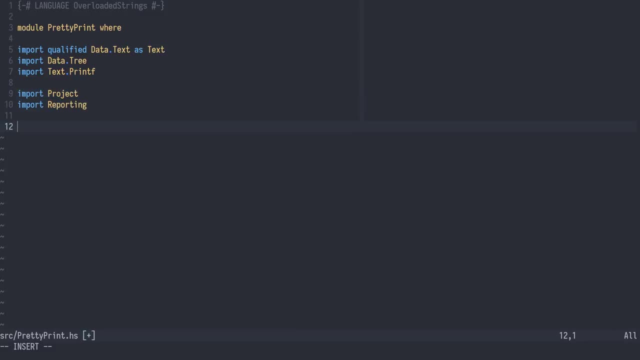 We also need our project and reporting modules. Now we can write asTree a function from project to a tree with string labels. We pattern match on the project and, given a single project, we will create a graph node where the label is produced by printf. 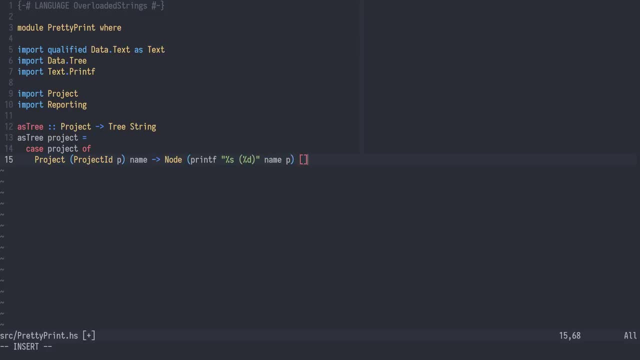 If we have a group of projects, we will create a node where the label is the name and the list of children is the mapping of asTree over projects. The PrettyProject function is a little helper, which is just the composition of DrawTree. 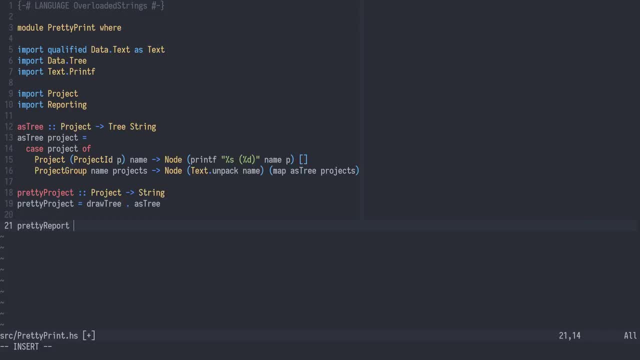 from DataTree and our asTree function. PrettyReport is a function from a report to a string. It's defined using Printf, creating a string with the budget, the net profit and the difference. We need to pick out the double values from the money for all three fields. 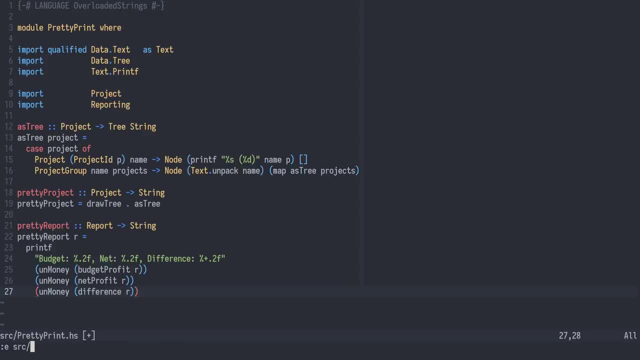 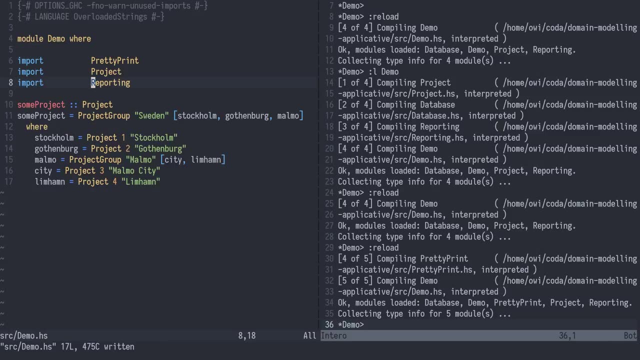 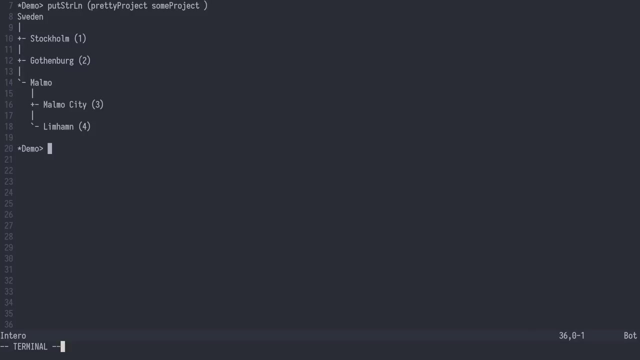 Going back to the demo module, we can import our PrettyPrint module and load this up in the REPL. We can print the Pretty version of a project like so, and we can calculate the project report and print that using the PrettyReport function. 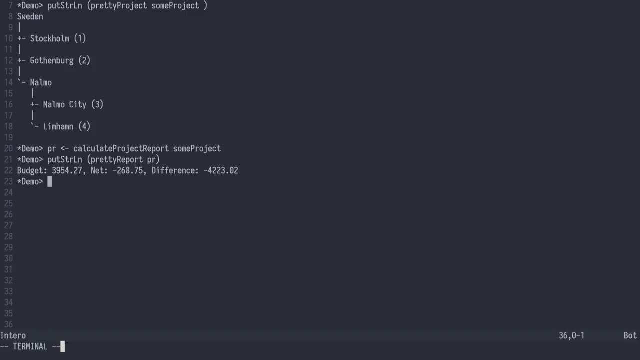 And that is it for this video. Thanks for watching. In the next episode we will see how we can generalize this using functor: traversable and foldable.